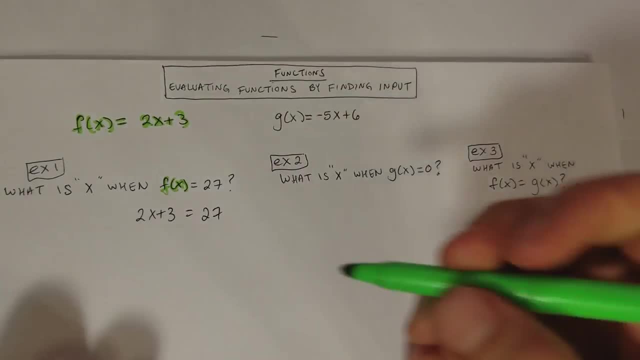 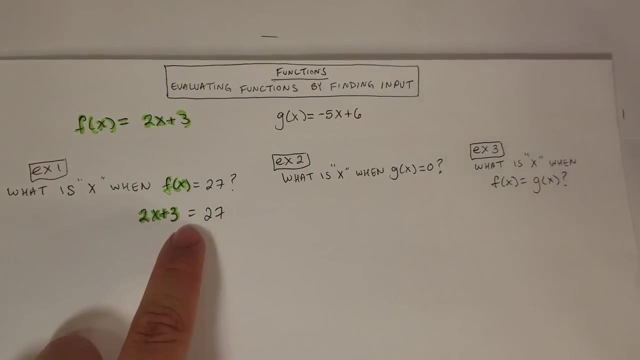 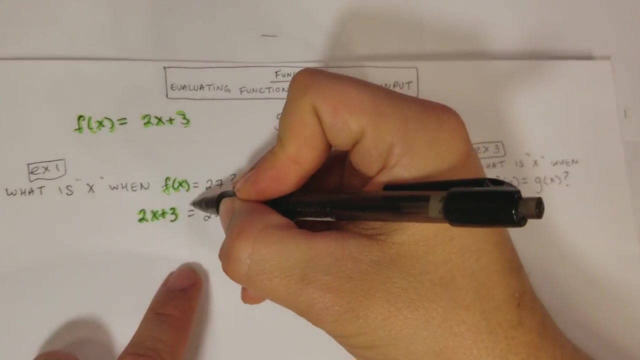 plus 3 equals 27.. And then could you find x if I set this function to 27.. Well, you better, because you should be familiar with solving linear equations by now. so it's basically what we've done before in this class. So you would basically draw the wall, Subtract 3 on both sides, minus 3, minus 3.. We get 2x on this. 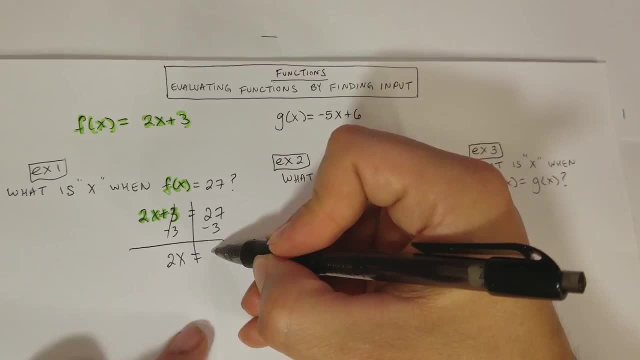 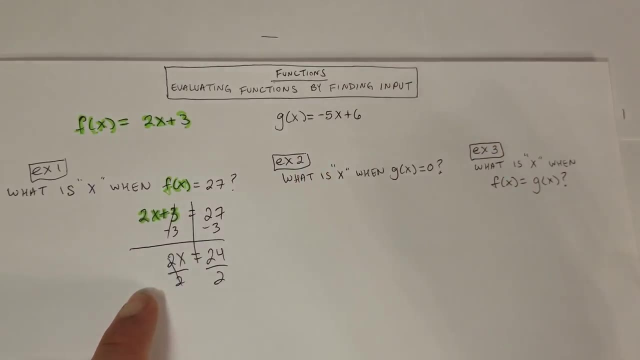 side is equal to 27 minus 3, which is 25.. Wait, 24, just kidding. Divide by 2 on both sides And then you get your final answer for x, which x is equal to half of 24, or 24 divided by 2, which is 12.. 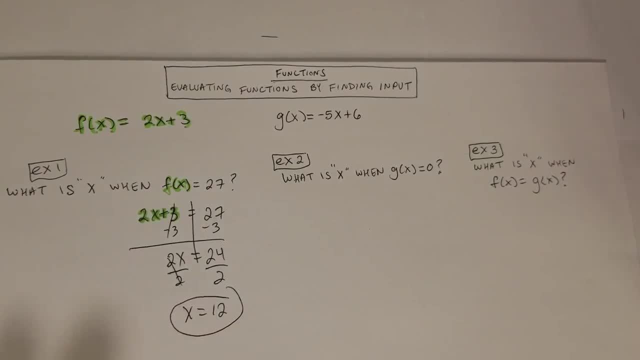 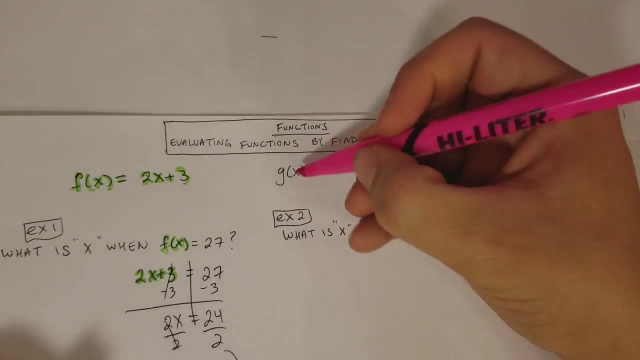 Bam. So example number one is done. So I hope it makes sense what we're doing. So if f of x equals 27, then the input or the x is equal to 12.. Let's do another one. So this time we're going to have function g of x, So function g of x is equal to negative. 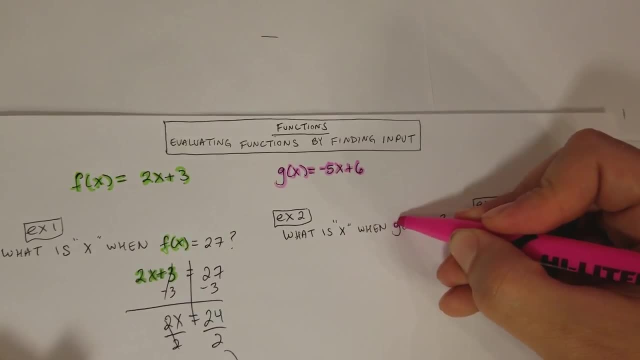 5x plus 6.. What is x when g of x equals 0?? So what we're doing here is we're basically setting the g of x equal to 0.. So I'm going to replace g of x with negative 5x plus 6. 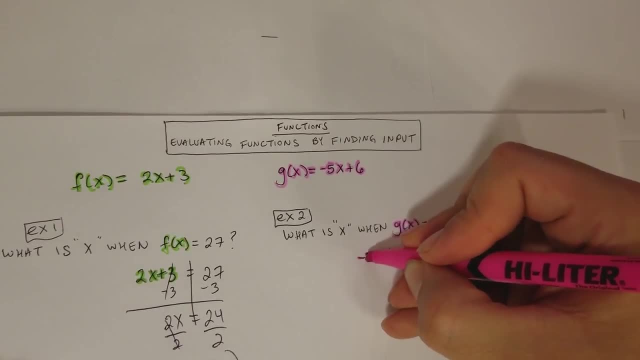 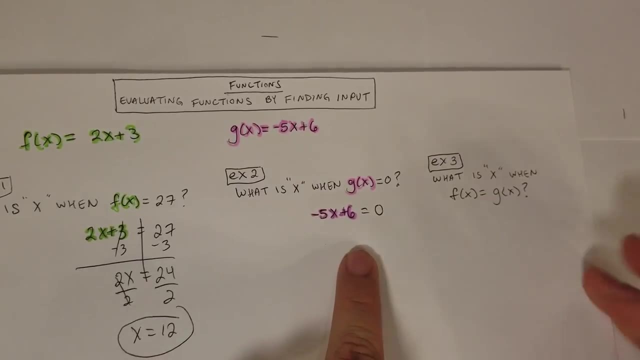 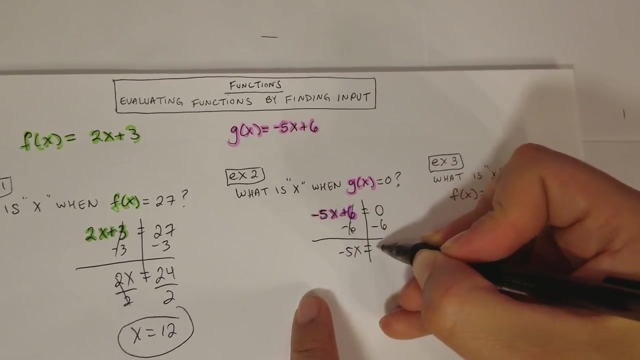 and then set that equal to 0. to see what we get for x 6, set it equal to 0. Solve Again. we've done this before, So we draw the wall. I know the equal sign: Subtract 6 on both sides minus 6, minus 6.. Negative 5x is equal to negative 6.. 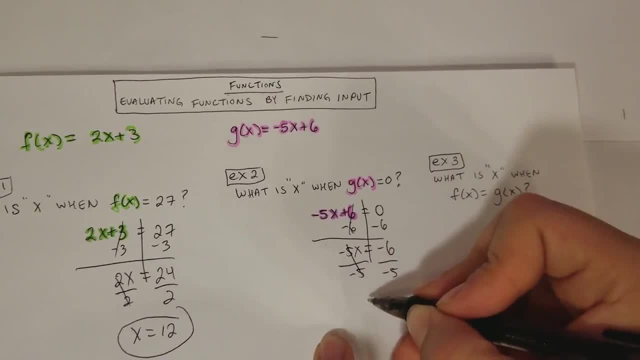 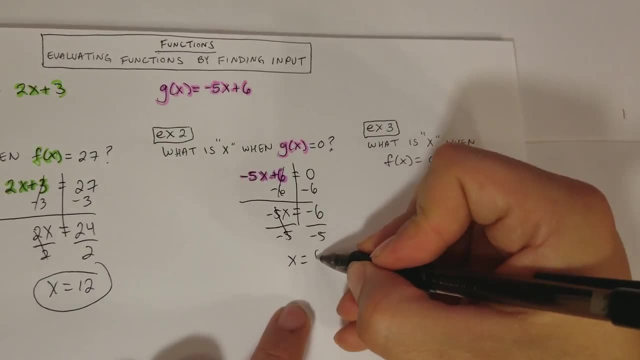 Divide by negative 5 on both sides: Negative 5, negative 5. We get: x is equal to negative 6 over negative 5. Notice that the negative over the negative actually cancel out. So we're left with just 6 over 5.. And again, leave it as a fraction. I rather deal with fractions of decimals. 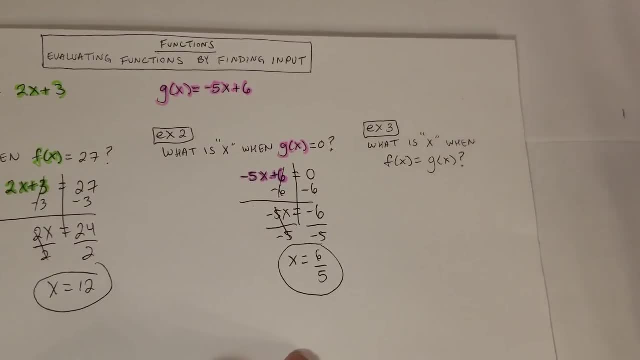 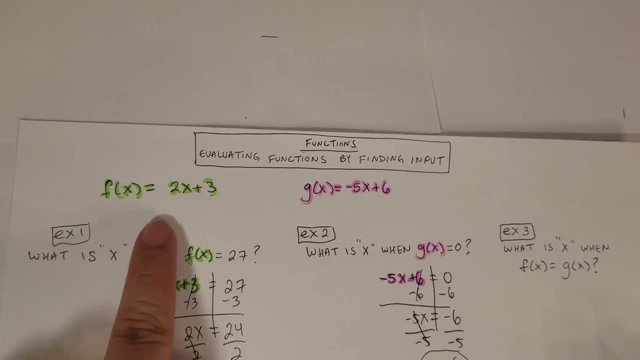 over the decimals, So you can leave it like that. Last example, So example number 3.. It says: what is the value of x when f of x equals g of x? So we have f of x, We have g of x. This is telling me to set them equal to each other. 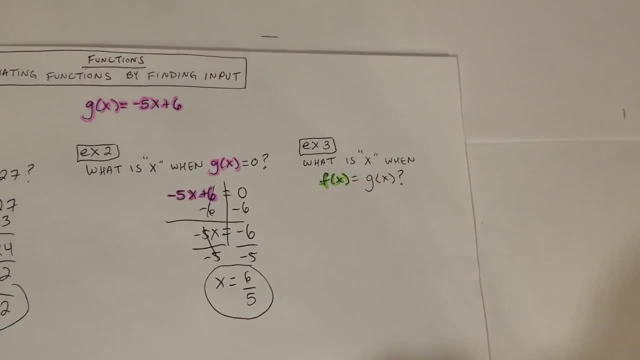 So basically, what we're doing here is we have f of x from the original problem and we have g of x from the next one. the next function Set them equal to each other. See what we get for x. So I'm going to do just that. So we're going to get 2x. 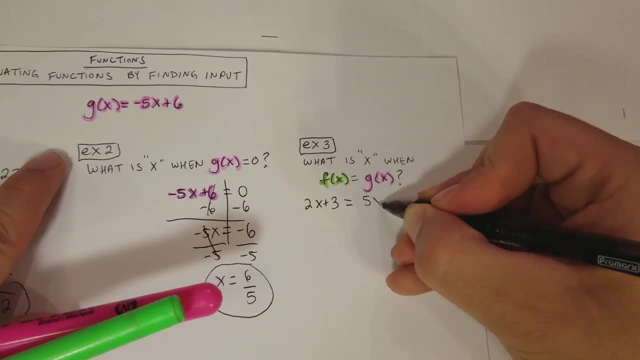 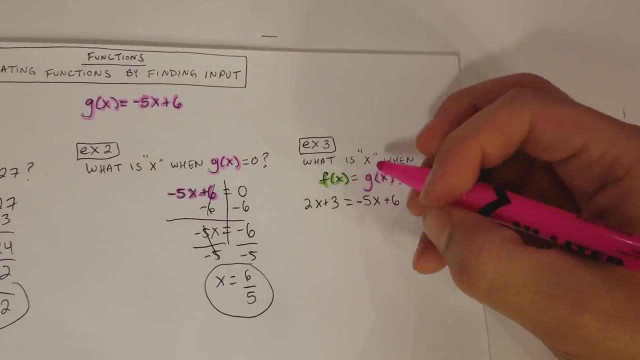 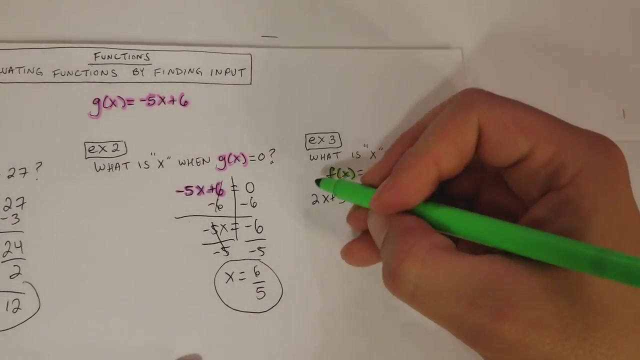 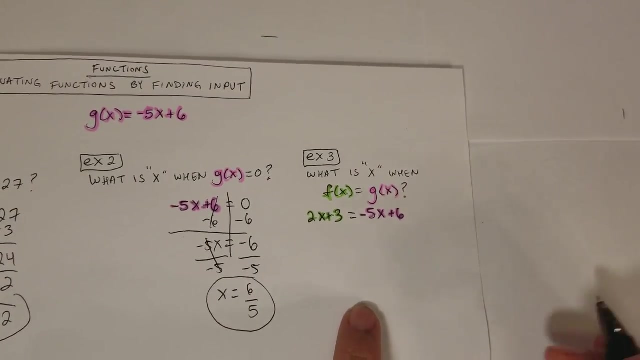 x plus 3 is equal to 5x plus 6, so that's actually negative 5x plus 6, if I plug it in correctly. So just to color code it, that was corresponding to the pink and then this was corresponding to the green. So solve for x Again. you've done this before, If you. 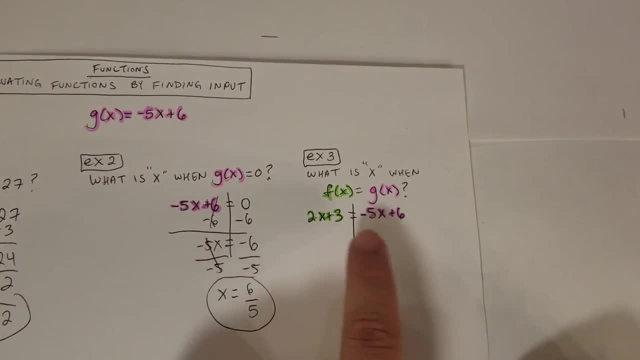 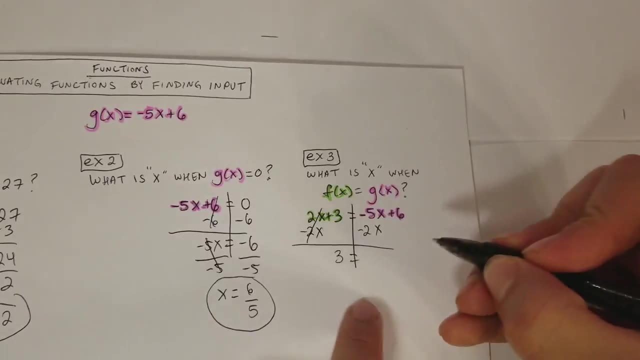 solve for x. typically you draw the wall, you move the smallest variable to the other side. In this case we subtract 2x on both sides. minus 2x minus 2x, We're left with 3. on this side is equal to negative 5 minus 2 is negative 7x, and then drop the 6 down. 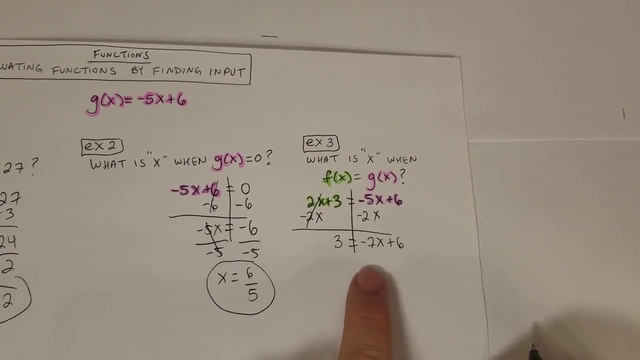 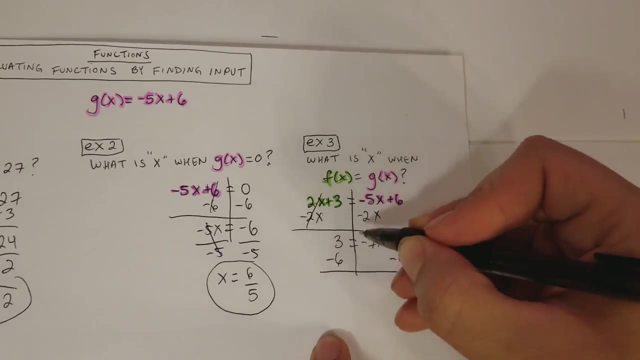 We're almost got the x by itself. so now we just got to get rid of the 6,. we got to get rid of the negative 7.. Let's start with the one that's furthest away, always. So subtract 6 on both sides, and then this goes away. We're left with 3 minus 6, which is negative. 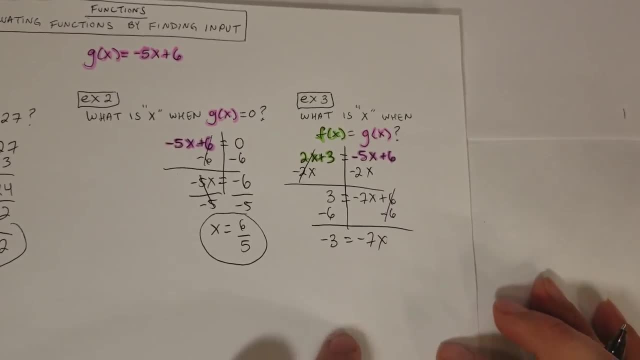 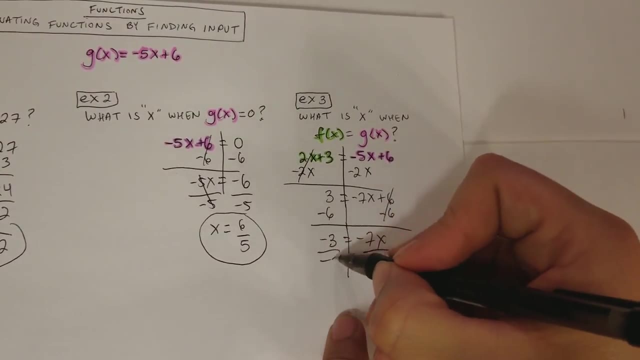 3. On this side we get negative 7x. Almost Almost done One more step. So we want to get rid of the negative 7, to get the x by itself. so we're going to divide that. So divide by negative 7, divide by negative 7,. 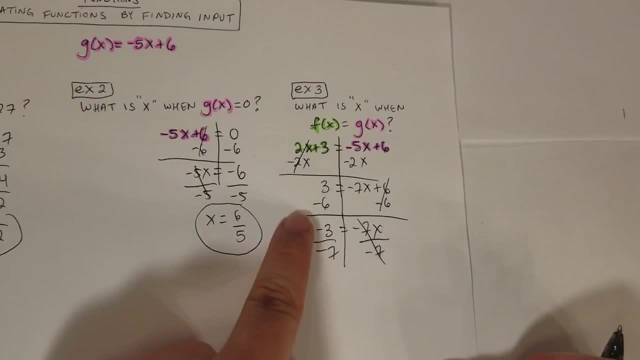 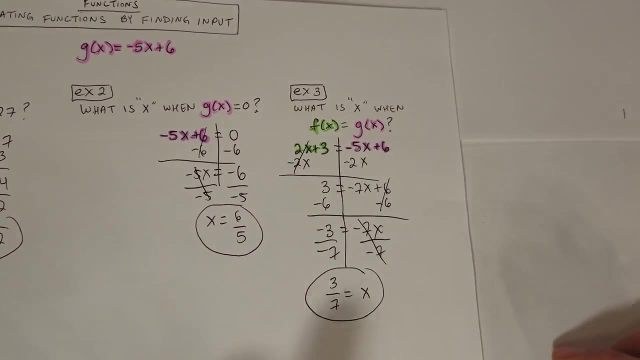 and we are done. So x is equal to that stuff. The negative and the negative cancel, so we get 3 over. 7 is equal to x. Boom, Don't be scared if you get fractions. Fractions are answers as well, so it doesn't mean that you did it wrong. If you follow the steps, you